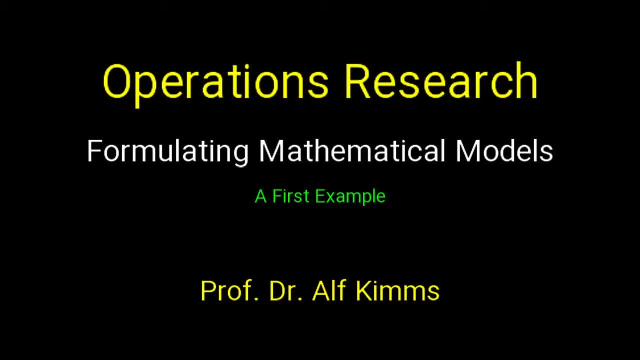 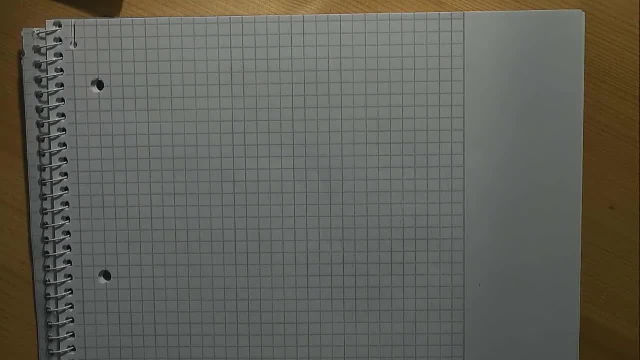 Modelling is a basic skill in operations research. but beginners often find it difficult to formulate a mathematical model. Hence I have decided to make a series of short videos in which I, step by step, explain how to model. You will see that modelling is indeed an art There. 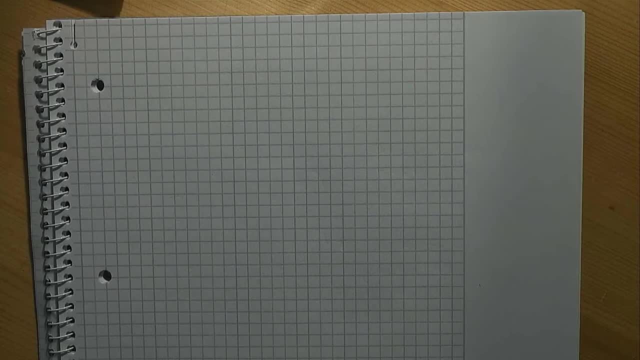 is no simple recipe to follow. Beginners should therefore not be frustrated when first attempts are tough. Just don't give up too early. You will learn by your mistakes Without further ado. let's have a look at the very first example. Suppose we want to. 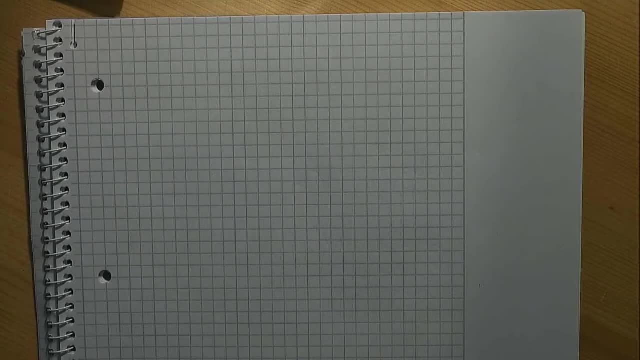 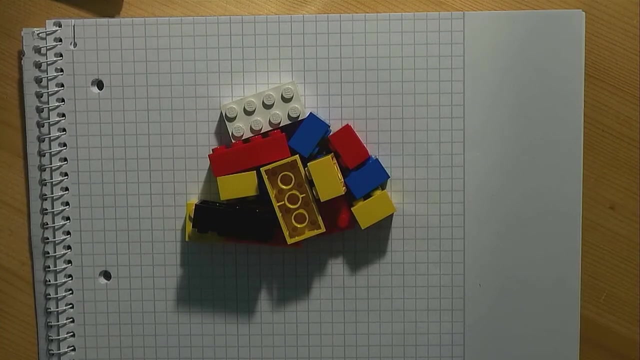 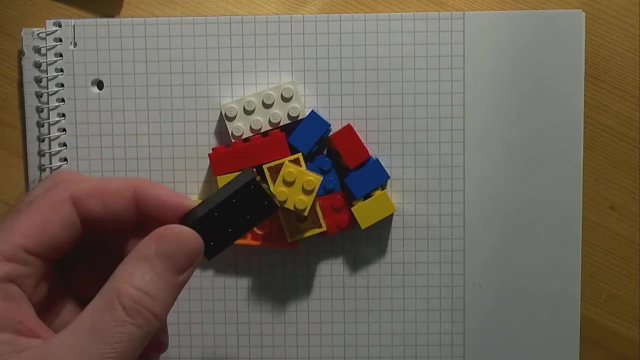 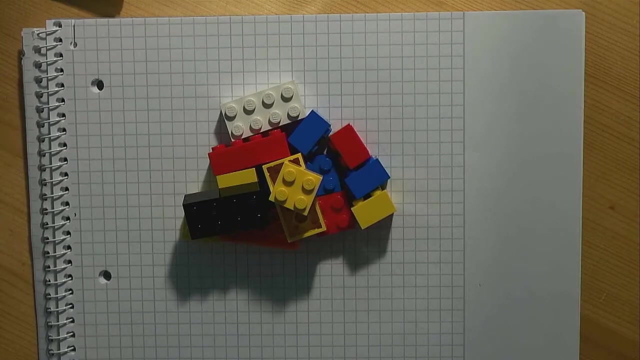 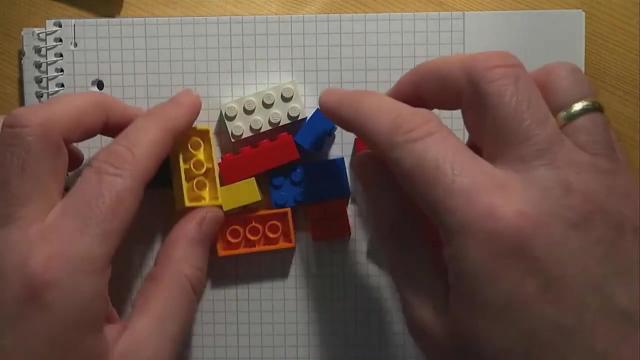 produce furniture from small wooden parts. To illustrate the situation, I have here a bunch of Lego bricks that represent those parts. As you can see, there are different kinds of parts. We have 2x2's and we have 2x4's. The number of parts is limited. We've got 8 2x2's and 6 2x4's. 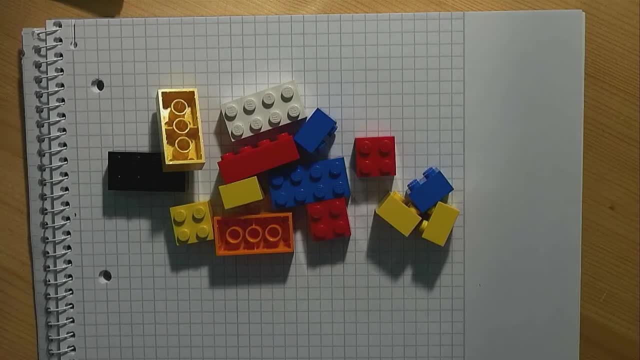 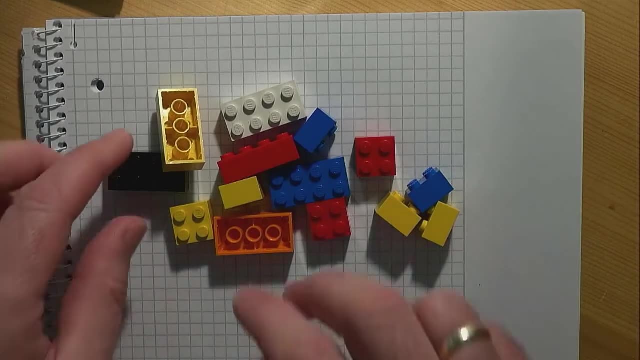 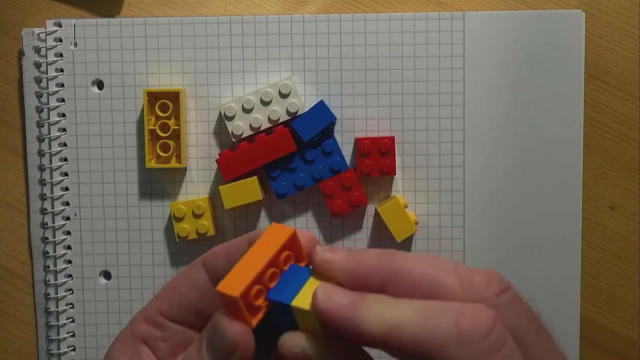 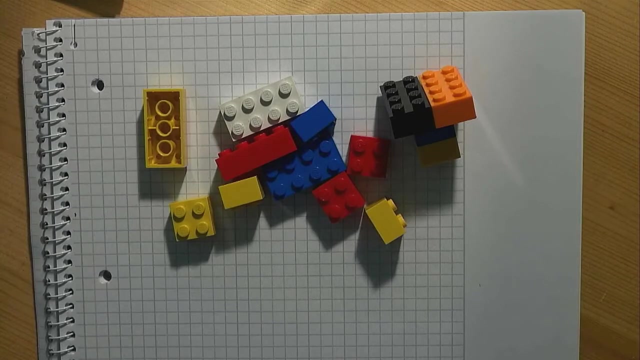 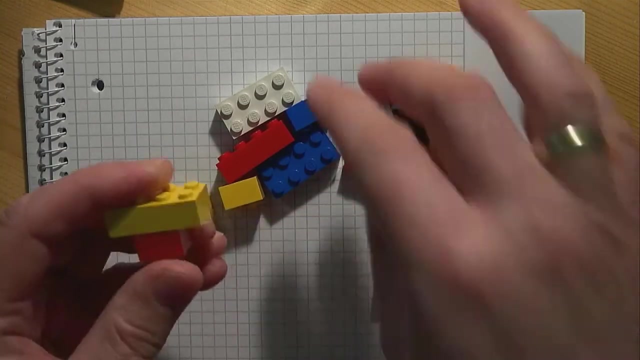 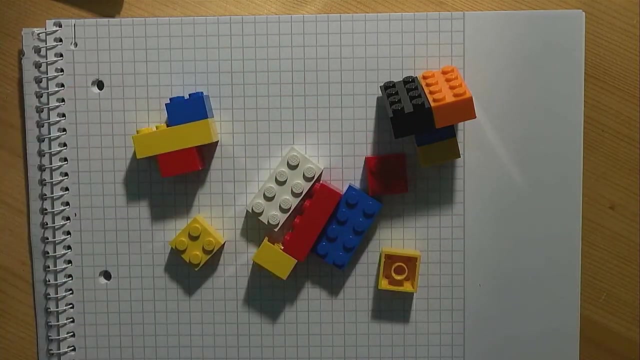 From these parts we can produce tables and chairs. A table is made out of two 2x4s and two 2x2s, like so A chair requires one 2x4 and two 2x2s. As an exercise, you should pause the video now to make a list of all possible combinations. 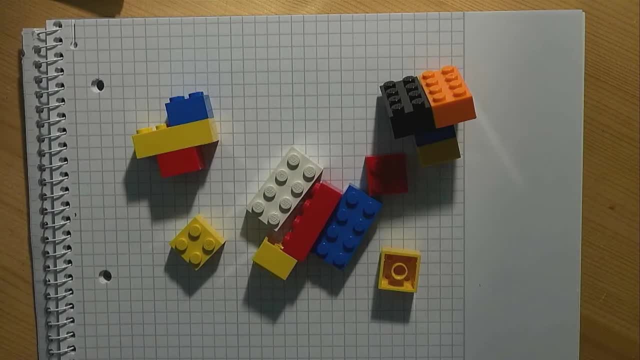 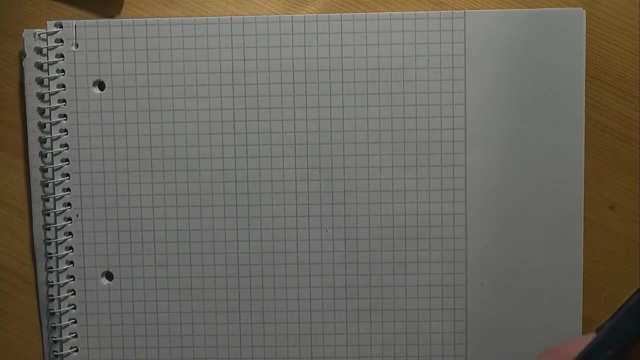 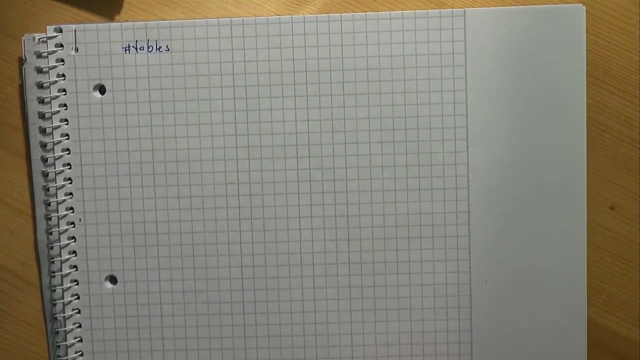 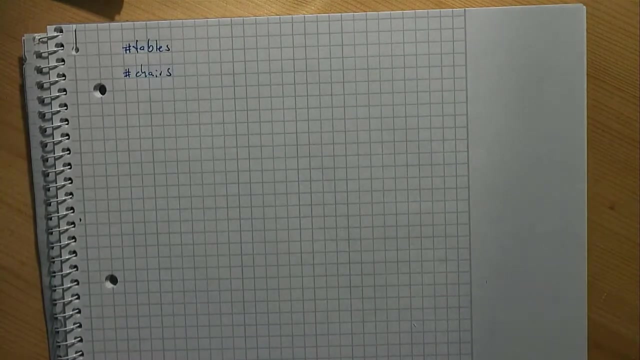 of tables and chairs that you can produce out of the parts that are available to us. Pause the video now. Your list may look like this: We have the number of tables and we have the number of chairs, So it is possible to produce three tables and no chairs. 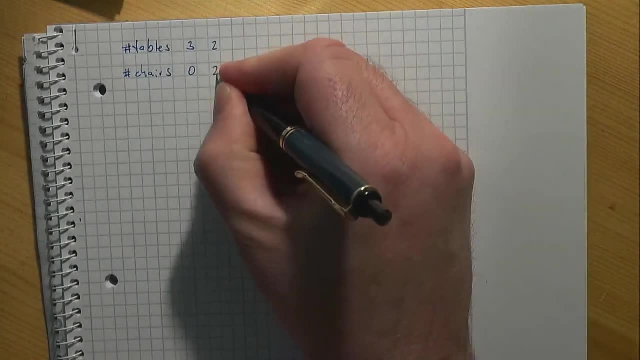 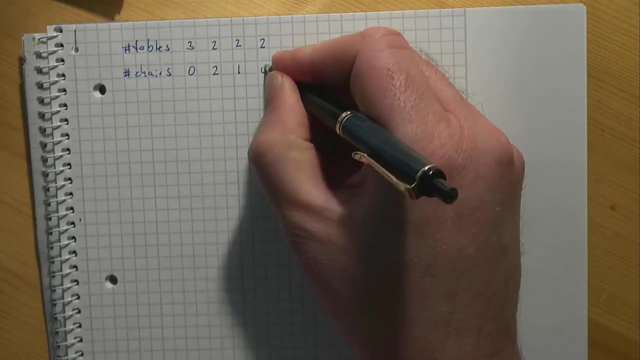 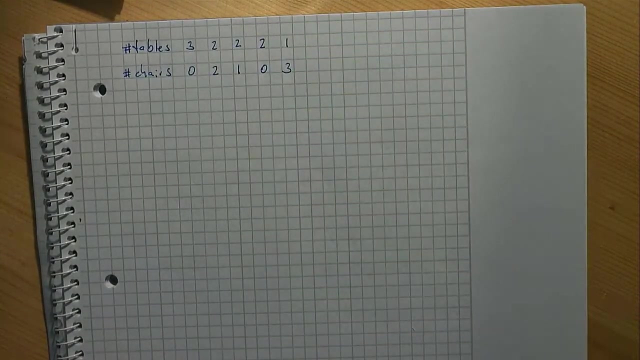 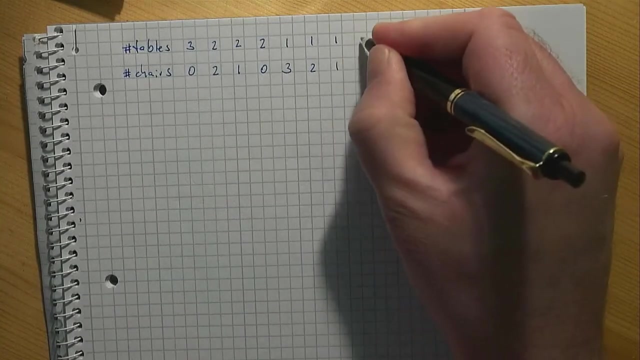 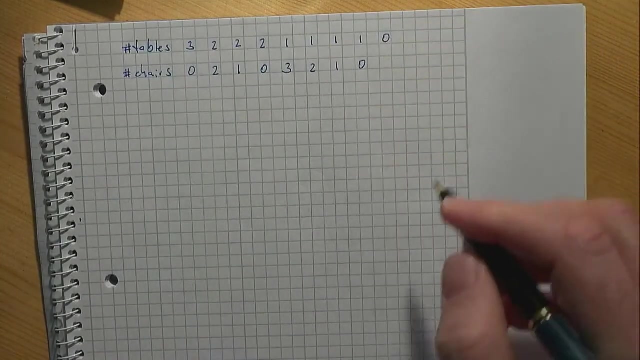 Also two tables and two chairs are possible. Two tables, one chair, Two tables no chair. Okay, we have one table and three chairs. One table, two chairs, One table, one chair, One table no chair. And also we have no tables and four chairs. 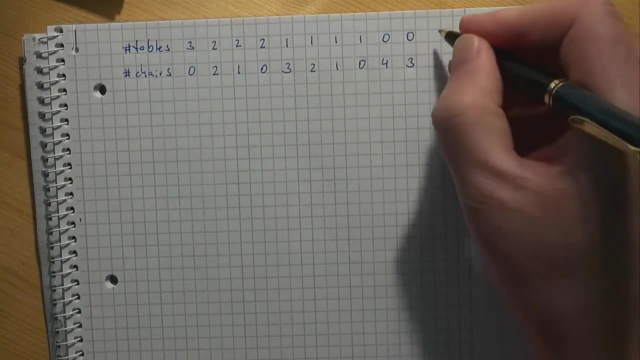 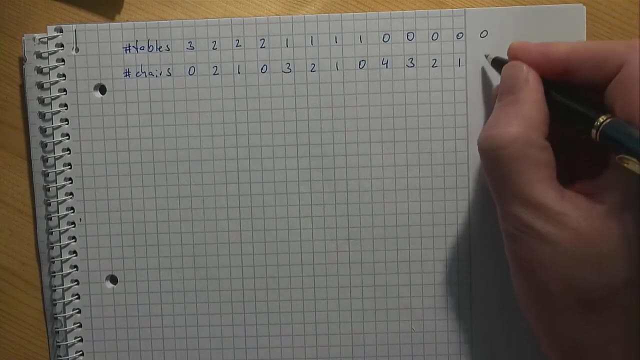 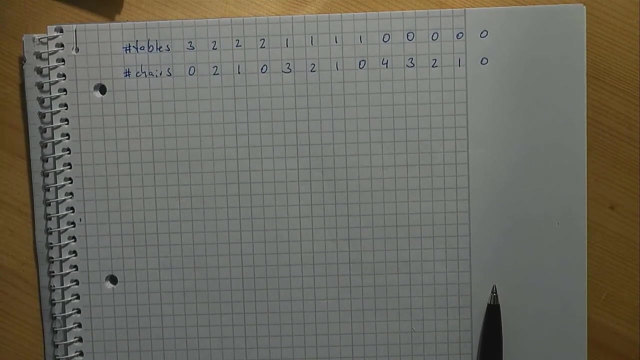 No tables, three chairs, No table, two chairs, No table, one chair Or no table and no chairs. Now let's try to model our situation. We want to know how many tables and chairs we should produce. This is unclear to us, and so we use symbols to represent those unknowns. 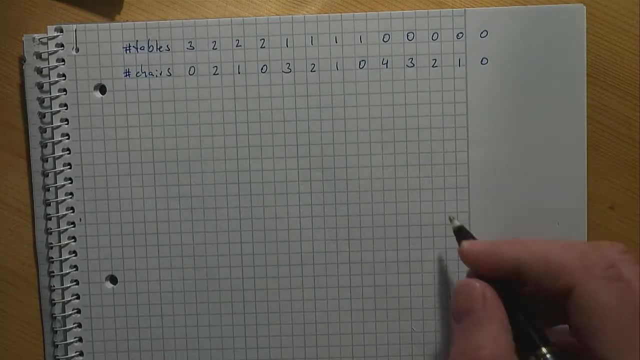 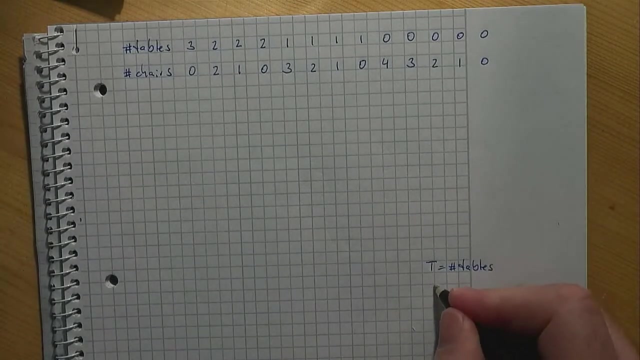 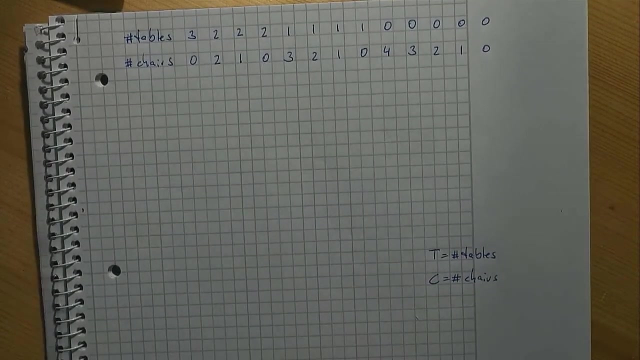 Let t be the number of tables And let c be the number of chairs. As part of the model, we usually specify the so-called numbers of chairs, So we can see how many tables we should produce And we can also see the number of chairs. 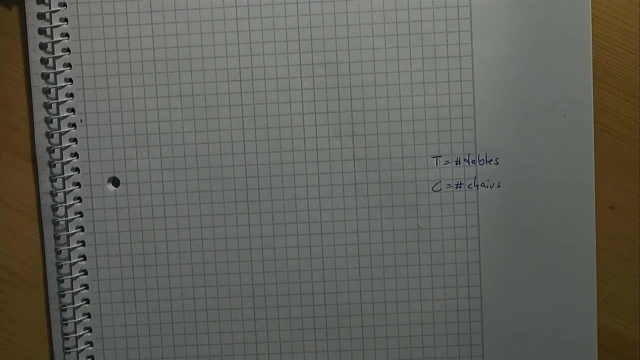 So we can see the number of chairs And we can also see the number of chairs. We usually specify the so-called domain of these unknowns, That is, the set of values from which we have to select a number In our application. we can define the domains as follows: 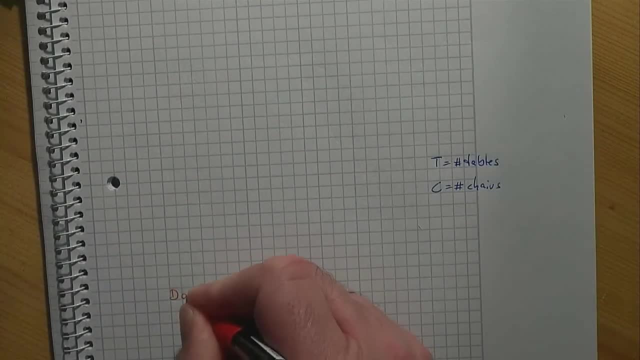 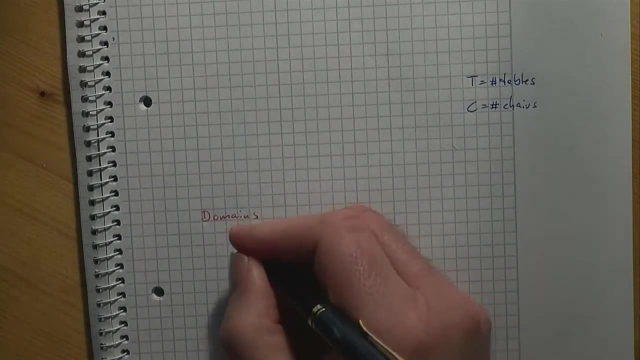 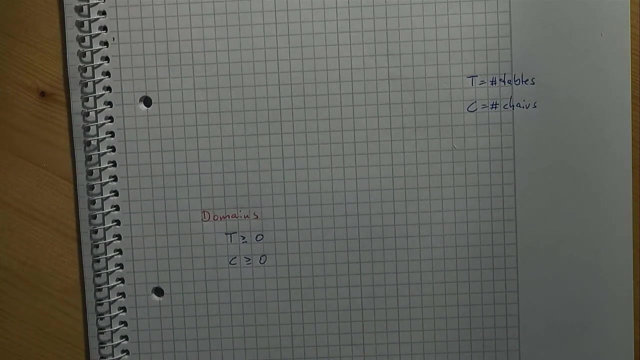 We can define: t is greater than or equal to zero. You can define: t is greater than or equal to zero, than or equal to zero and C is greater than or equal to zero. This makes sense because we cannot produce a negative number of tables or chairs. Note that it. 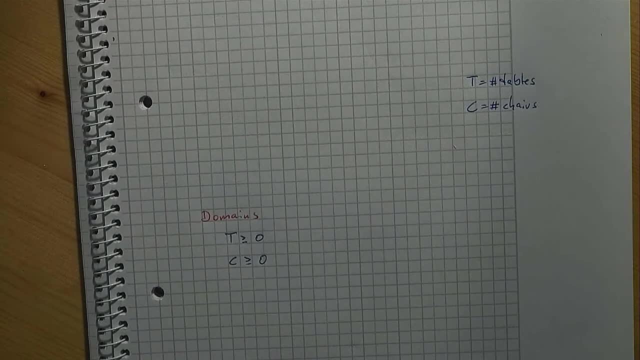 is common practice to have real numbers in mind, unless otherwise stated. This means our domain for T as well as for C, is defined to be the set of non-negative real numbers. For the time being, let's not worry about integers in this application. Next, we have to write down the conditions or the constraints, as we 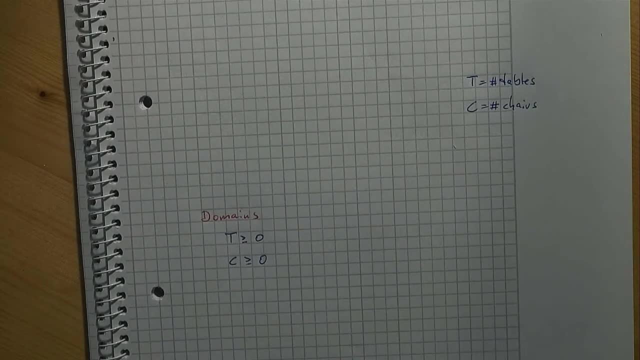 call them that we have to take into account In our furniture production problem. we have to take into account that the number of parts is limited For the two by fours. this means that we must not use more than six. Recall that we need two for a table and one for a chair. Formally, this can be written: 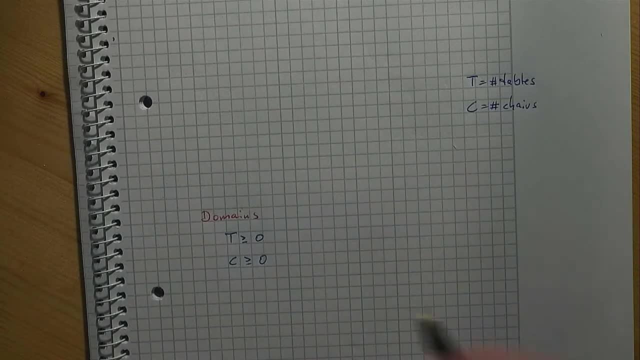 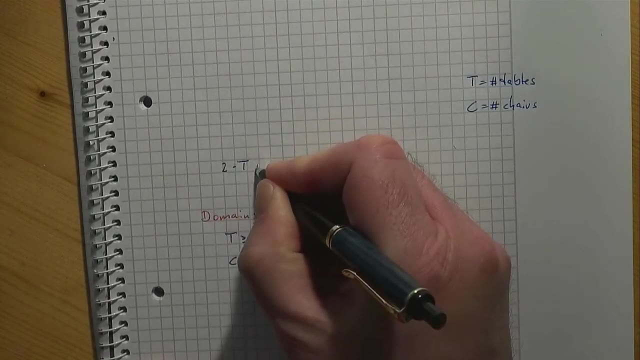 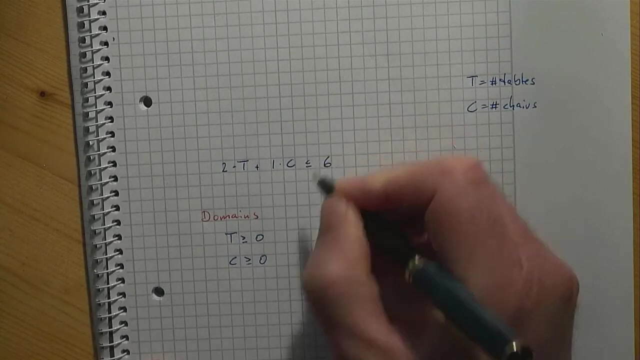 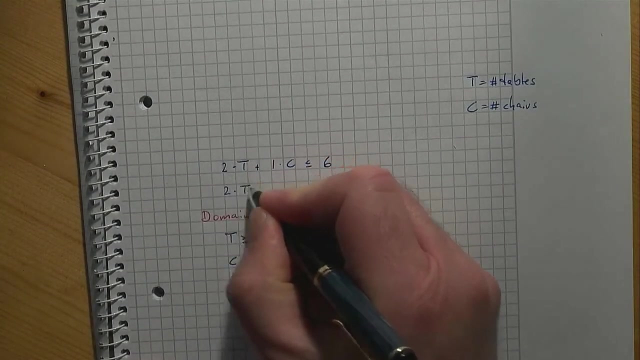 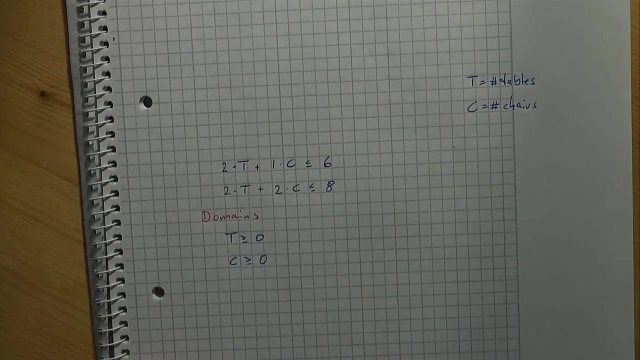 as follows: Two times T plus one times C is smaller than or equal to six. In a similar fashion, we have: two times T plus two times C is less than or equal to eight For the two by twos, because we have eight of them and two are required. 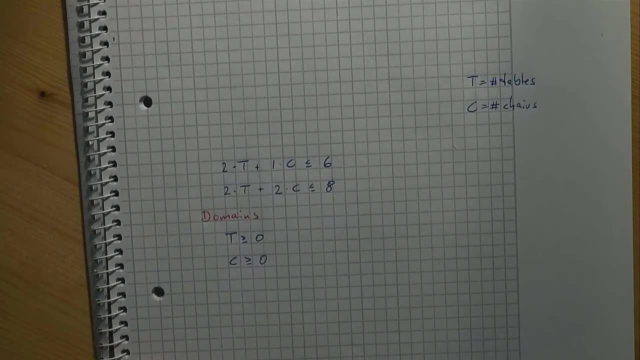 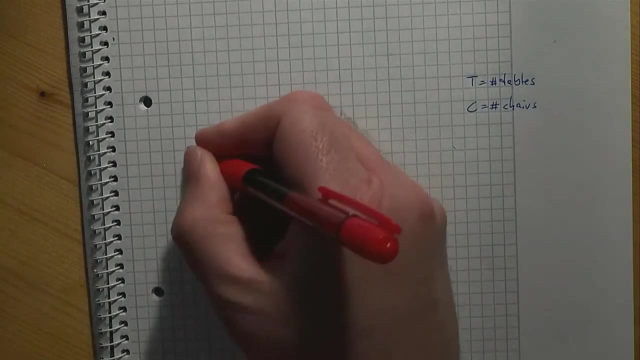 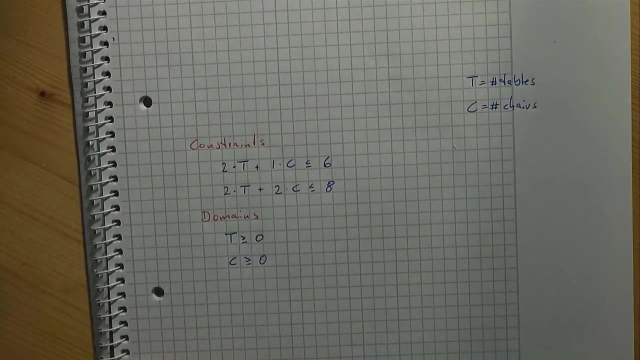 for each piece of furniture. By the way, the order in which we write down the constraints does not matter. what we have now is a very first model. that wollen wir jetzt. das erste Modell des the situation we had given A few technical terms, should be introduced at. 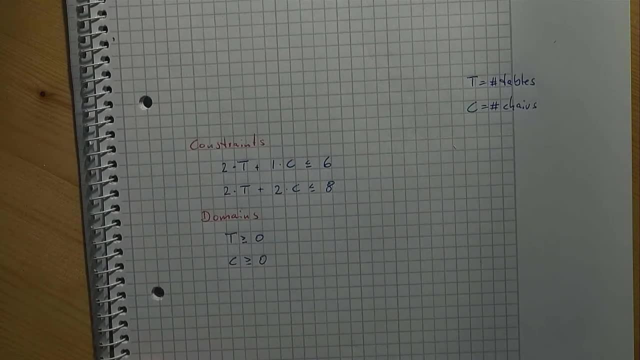 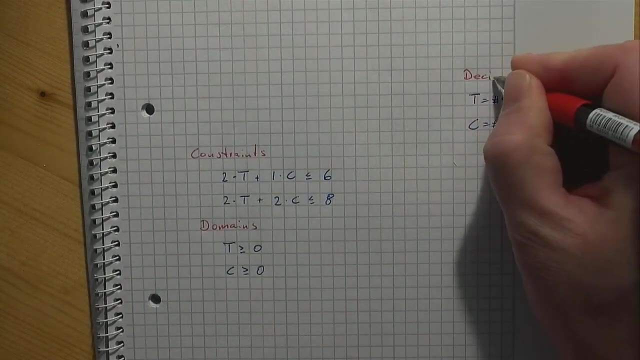 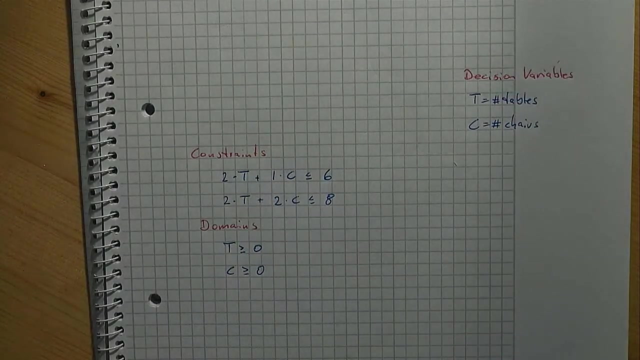 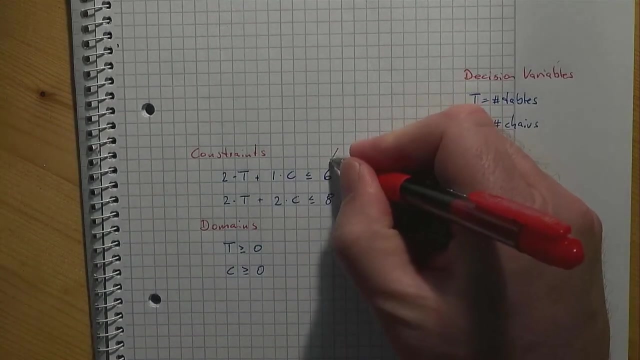 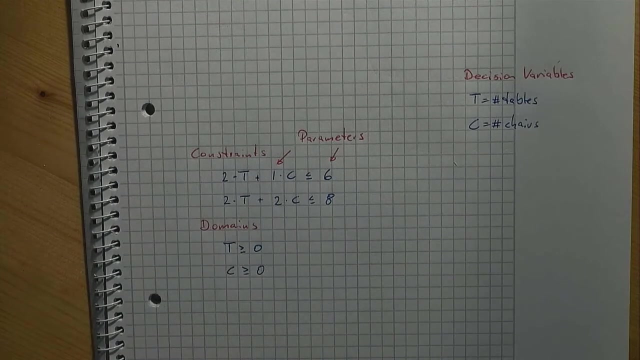 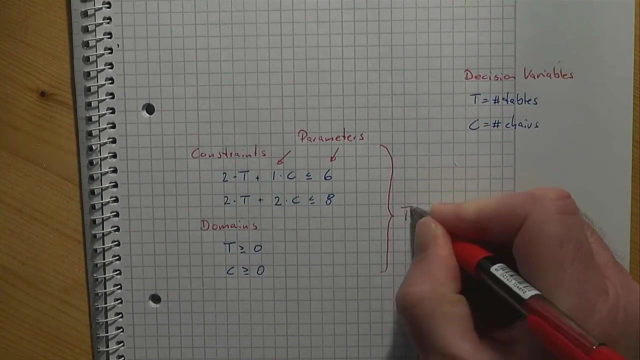 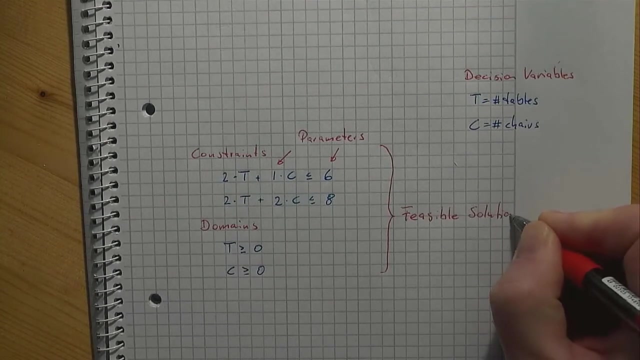 this point. The unknowns are referred to as decision variables And the data that was given to us is called parameters. A feasible solution is an assignment of values from the domain to the decision variables, such that all constraints are fulfilled without exception. Note that the list you have compiled contains all feasible solutions for our 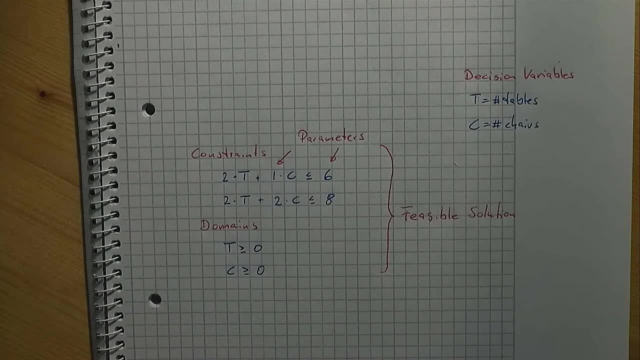 problem, given that we confine ourselves to integer solutions only, which is something we agreed not to worry about in this video. Let's now assume that we can sell the furniture that we produce. Suppose that the price for a table is 16 euros and the price for a chair is 10 euros. 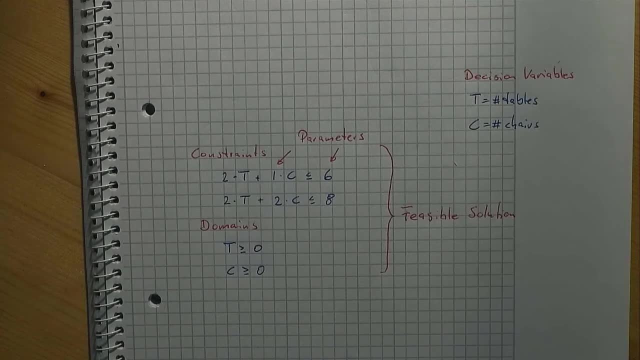 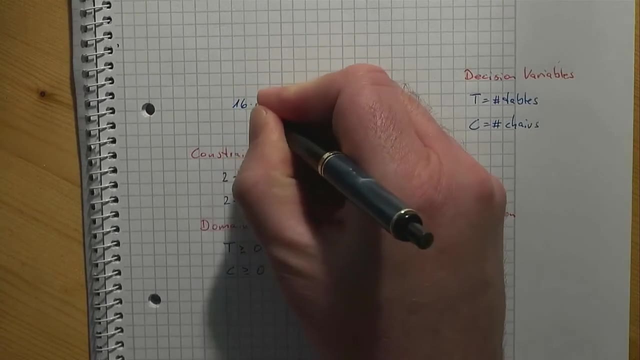 This leads us to what we call an objective function. Let's assume that the price for a table is 16 euros and the price for a chair is 10 euros. Let's assume that the price for a table is 16 euros and the price for a chair is 10 euros. 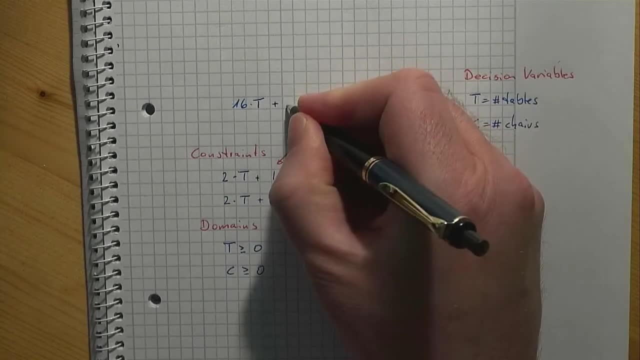 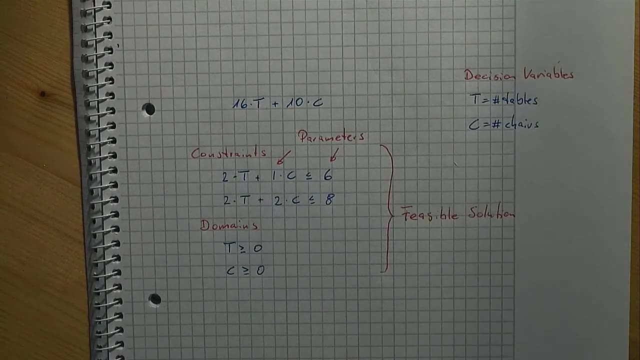 Let's assume that the price for a table is 16 euros and the price for a chair is 10 euros. The value of the objective function would be 16 x t plus 10 x c. That's the function that assigns a value to each solution. 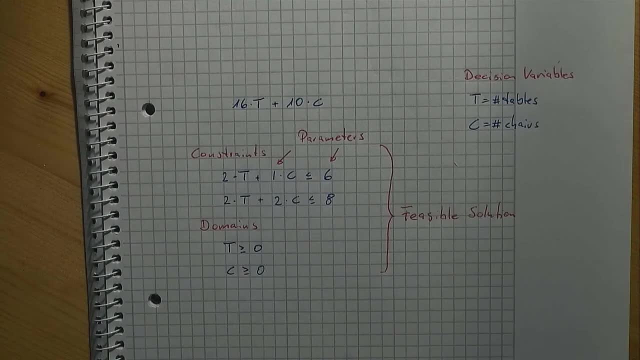 If we want to compare two feasible solutions with each other, we can now compute their objective function values and compare them. In our application, it might arrive at the following expression: might make sense to claim that the more money we earn, the better it is. 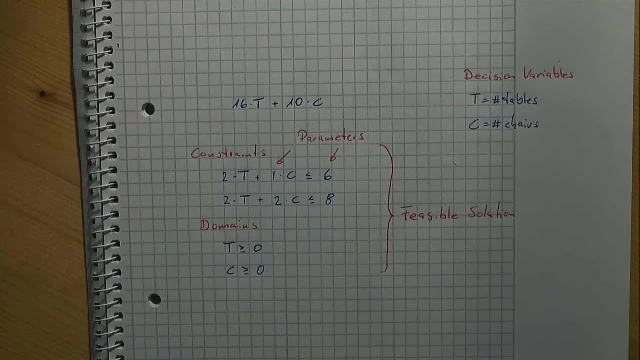 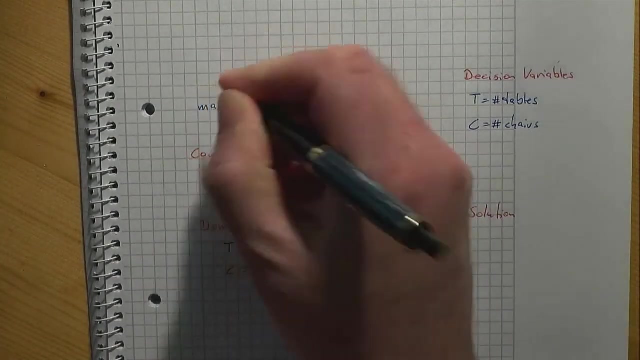 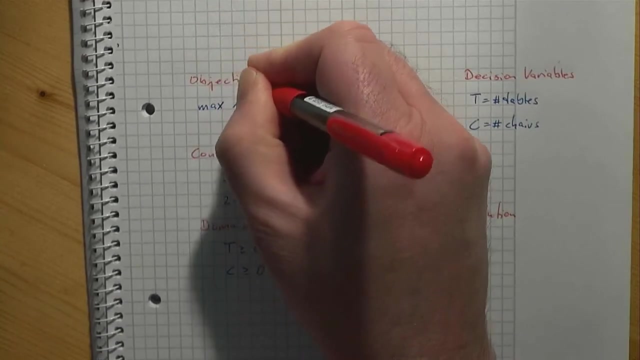 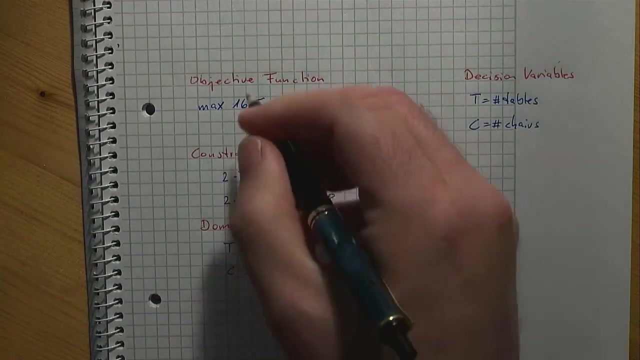 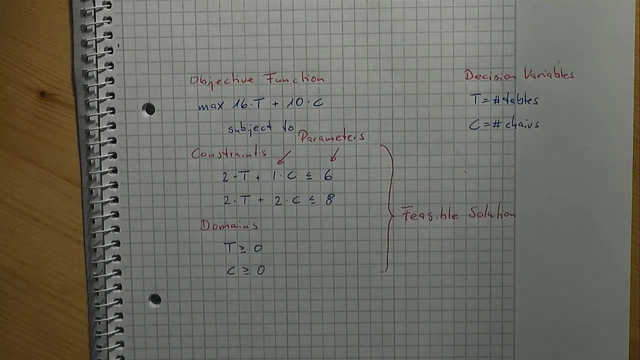 Consequently, we face a maximization problem. What is the number of tables and chairs that we should produce such that we earn the most money? Formally this is written like so In other contexts we may face a minimization problem and we would write min instead of max. then 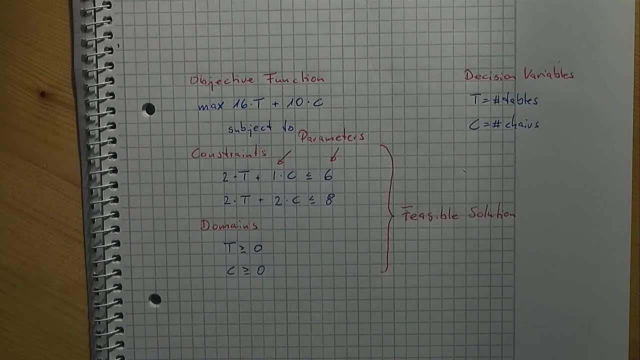 Note that the objective function does not have any effect on what is a feasible solution and what is not, But the other way around. only a feasible solution can be an optimum solution. An optimum solution is a feasible solution, such that the objective function value is best among the feasible solutions. 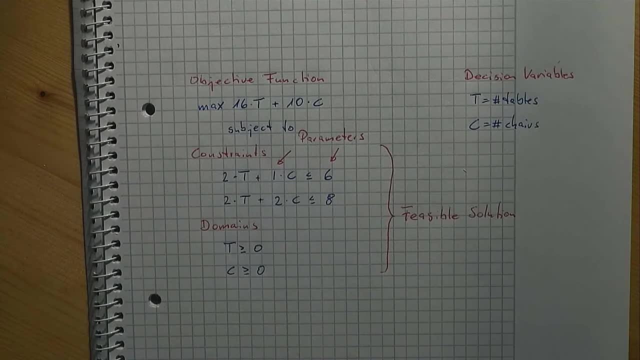 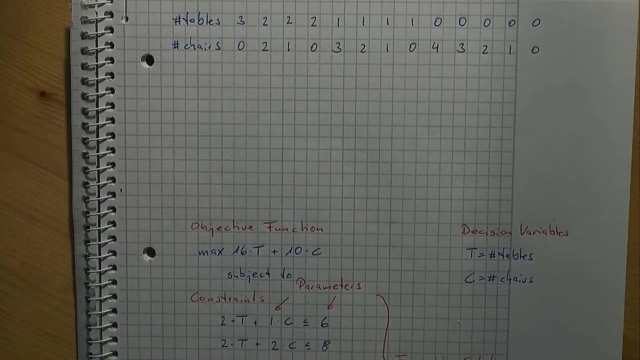 As an exercise, you may pause the video again and compute the objective function values for all the feasible solutions in your list. Find the best solution in our problem. Pause the video now. If you did right, you found that it is best to produce two tables and two chairs. 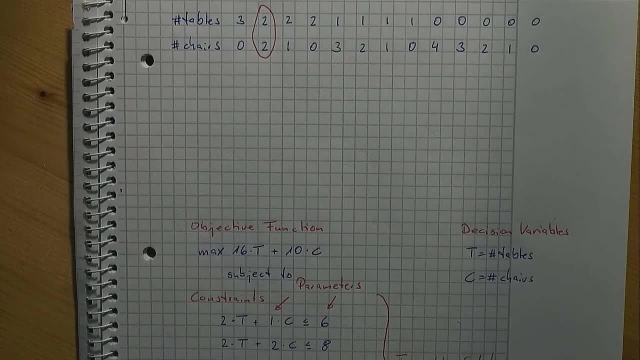 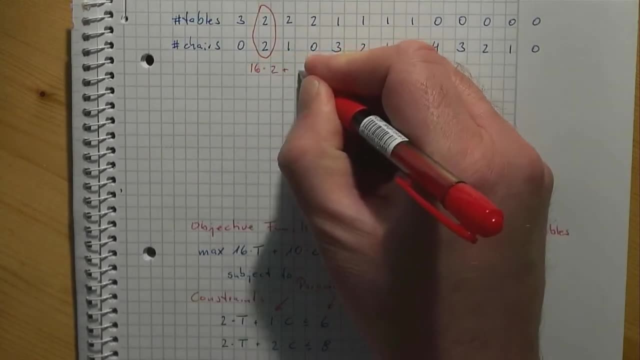 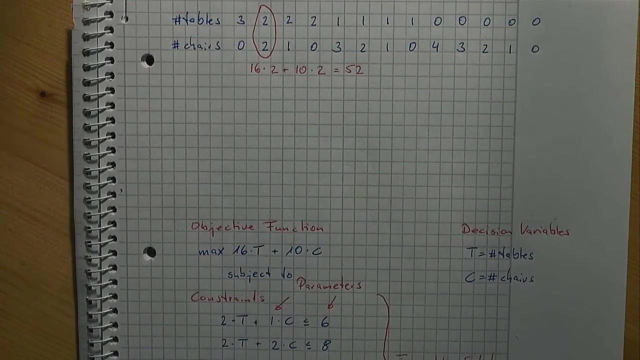 The optimum objective function value is 52 euros. Note that if you were asked to name a feasible or even optimum solution, you have to provide nothing more than values for all the decision variables. In our case, we would say that t equals 2 and c equals 2 is an optimum solution. 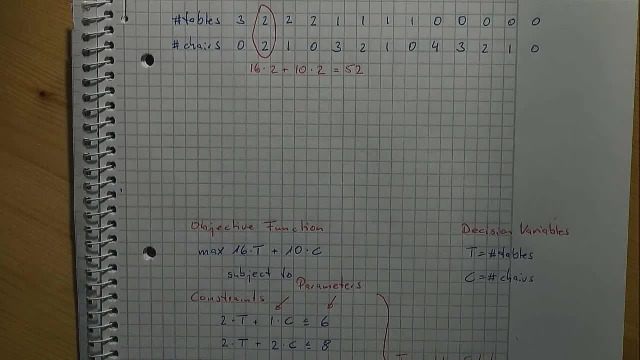 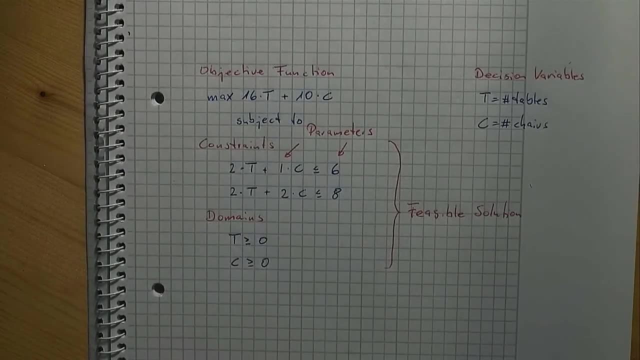 The corresponding objective function value 52 in our case is additional info. To wrap things up, let's recall what we have learned by this first example about the typical approach in operations. research First. there was a story producing furniture in our case. 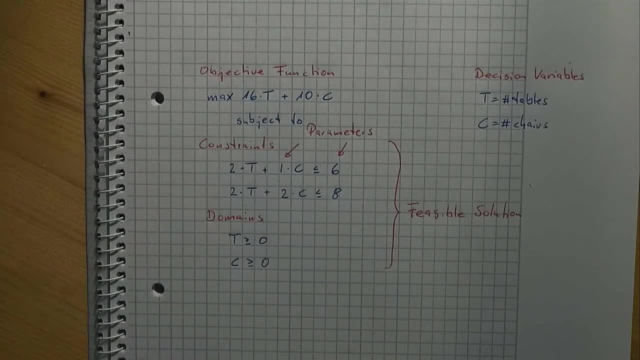 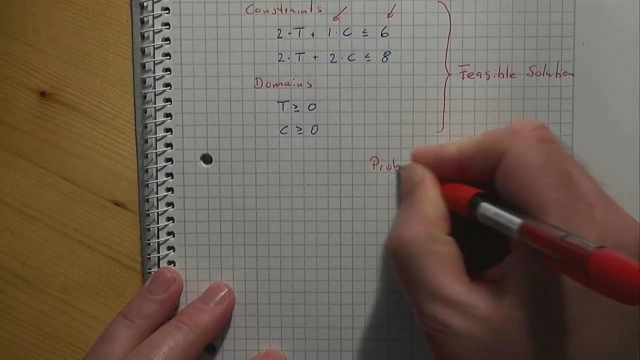 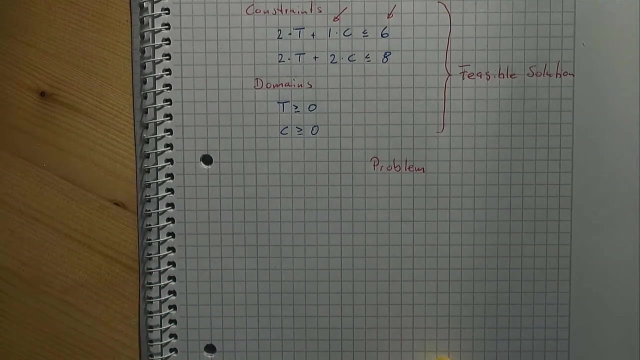 In operations research. this story is called the problem. We may face a feasibility problem. Any feasible solution would be fine. Or we may face an optimization problem. A solution with best objective function value is desired. Next we can describe the problem in mathematical terms. 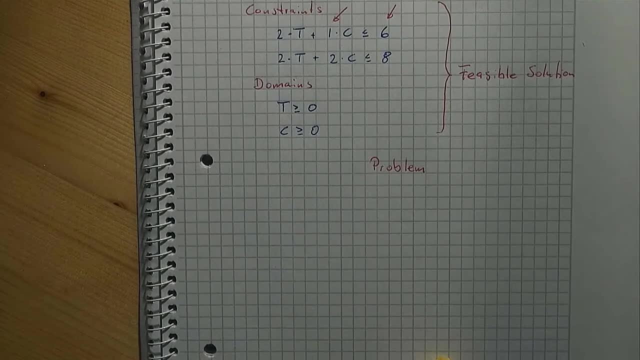 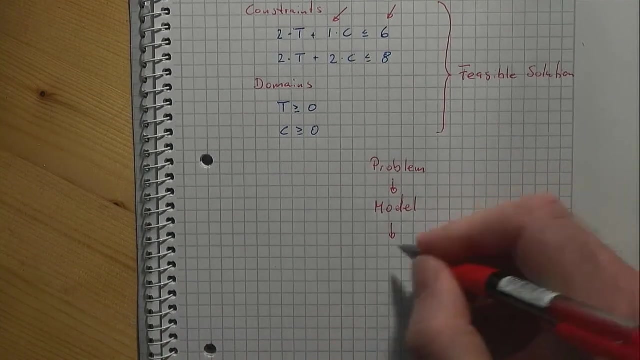 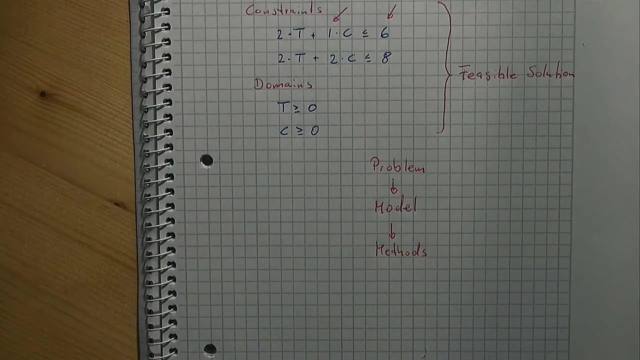 Parameters, decision variables and their domains, constraints and possibly an objective function. This is called a model. On the third level, we have solution methods. You have used a solution method that is called complete enumeration. You have listed all feasible solutions and you have selected the best one. then